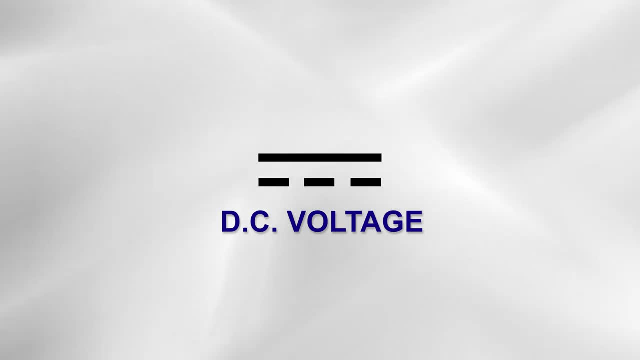 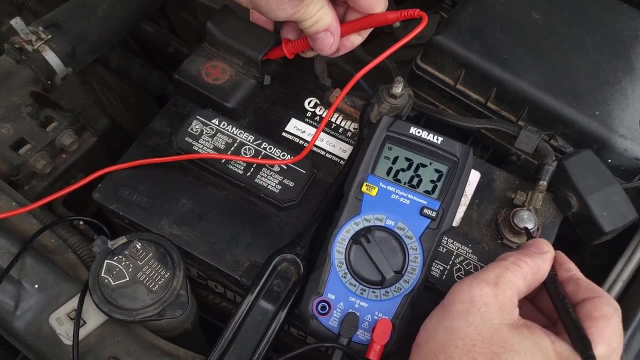 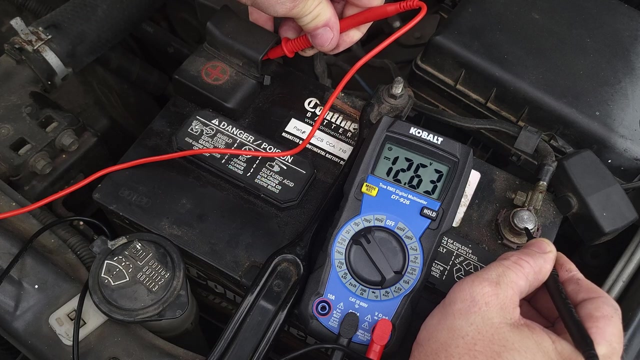 by the way, this symbol represents DC. So now we're going to put our black lead on the negative of the battery and then the red lead on the positive of the battery and, as you see, we get 12.63 volts. So this battery is good. Next we'll go inside and test some common batteries. This is a AA battery. 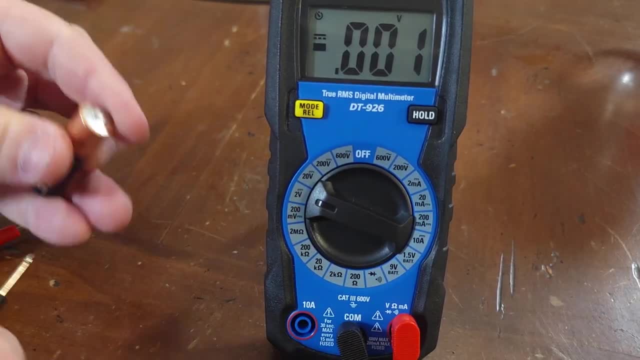 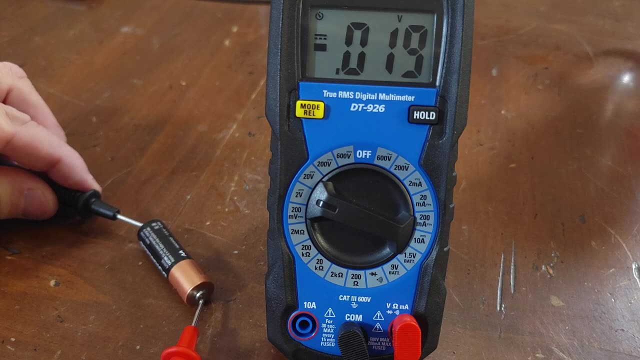 We'll put it on the 2 volt DC scale because this is a 1.5 volt battery And it looks like this battery is testing. this battery is dead: 0.019 volts. It should be 1.5 volts And I'll try another battery. 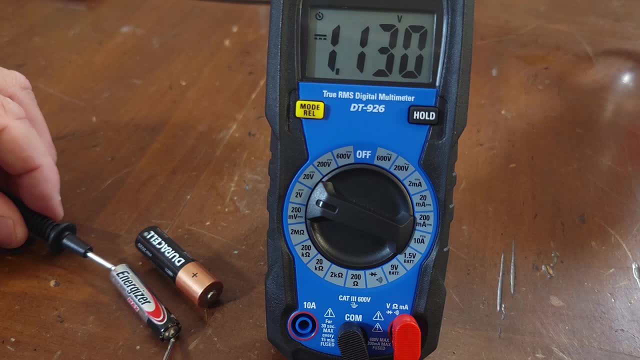 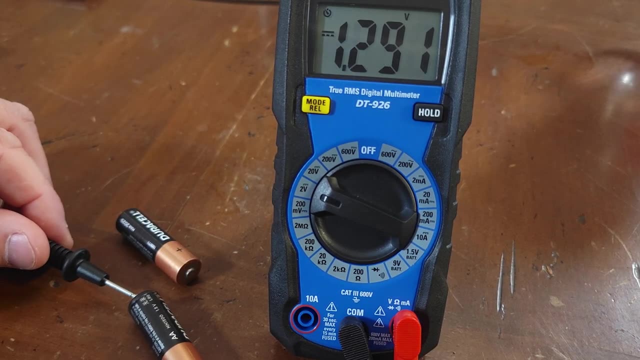 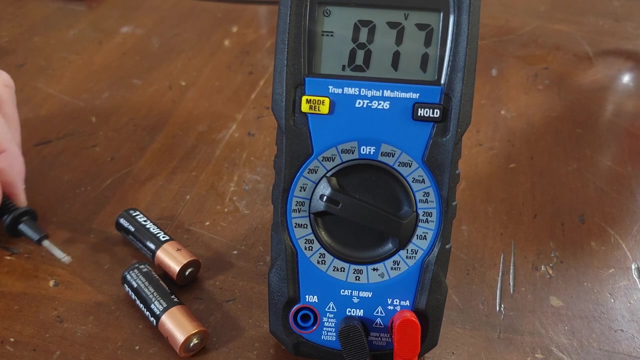 And this battery is low. It's 1.1 volts, A little bit closer, So I'll try one more battery. This battery is a new battery, 1.6 volts. This is what your AA does. should test like 1.6 volts or around that, because it is a 1.5 volt battery. 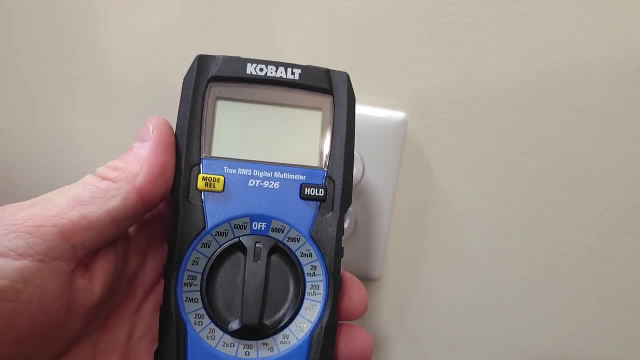 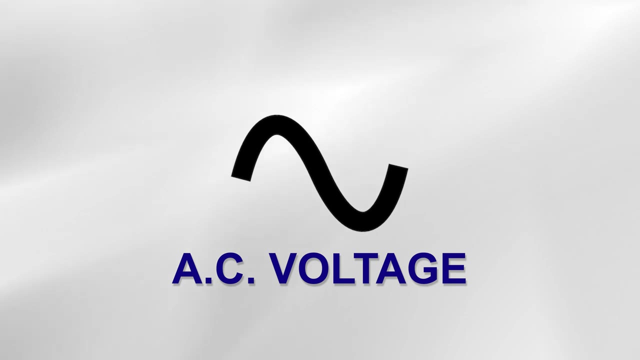 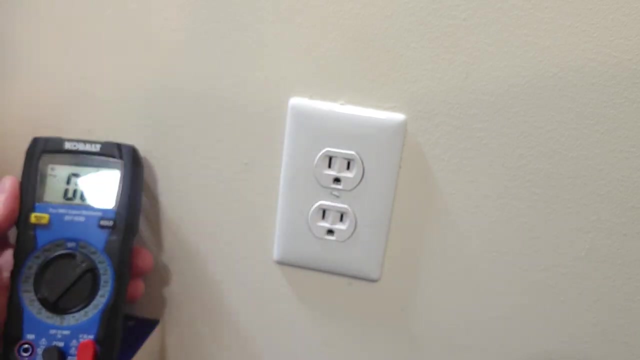 Next we'll test for household AC voltage. This should be about 120 volts, so we will put this meter on the 200 volt scale and this is the symbol for AC voltage. Now the next step is for demonstration purposes only. This could shock or kill. 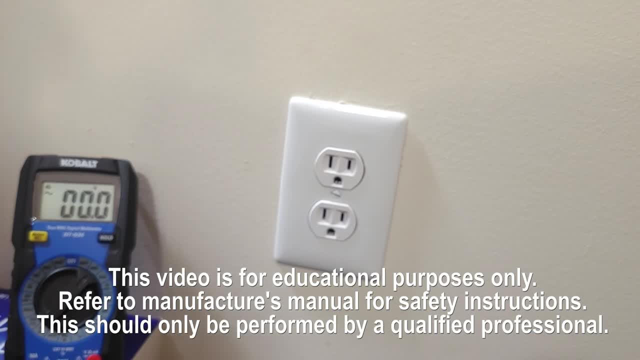 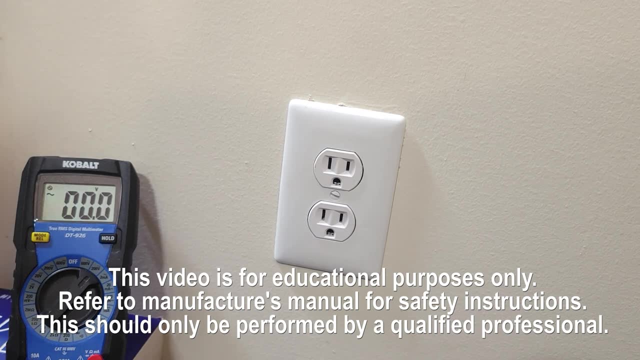 you if it's not done correctly. So always seek further safety instructions than this video. The wider blade on the outlet on the left is the neutral side. I'll put the black lead into it. I'll do that first and then put the red lead into the. 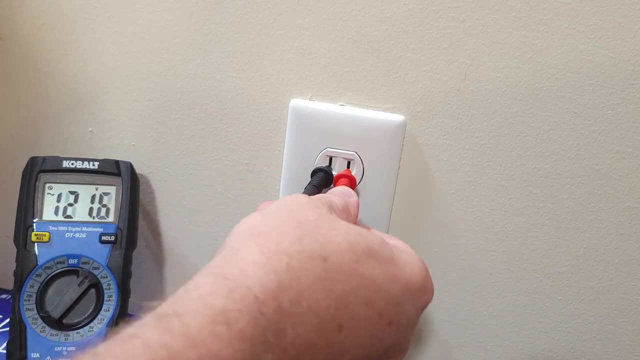 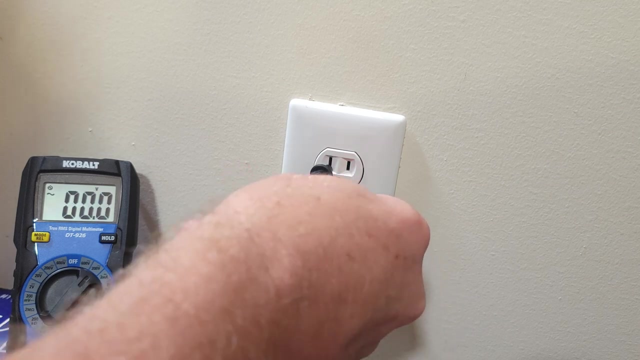 smaller blade, which is the hot side, and, as you see, we get 122 volts. Next we'll test the ground from the hot to ground. I've got 122 volts and then we can test from the hot to the hot side. The neutral to ground is 0 volts. Next we're going to test for resistance. This is the 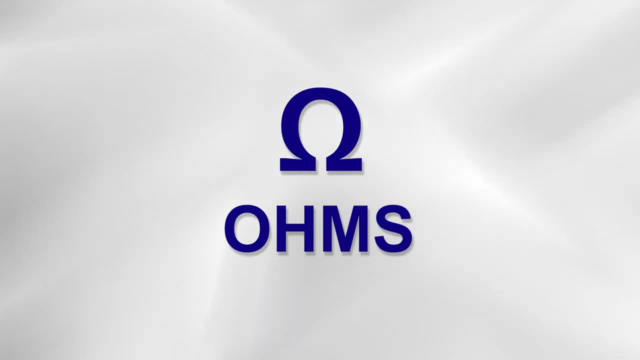 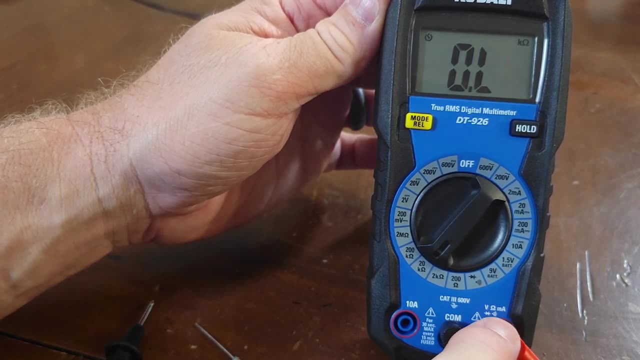 symbol of ohms, which is the standard unit of electrical resistance. The resistor we are going to test is 4.3k ohms, so I'll put it on the 20k ohms scale. and the meter leads are plugged in the proper place. The red is in the ohms.